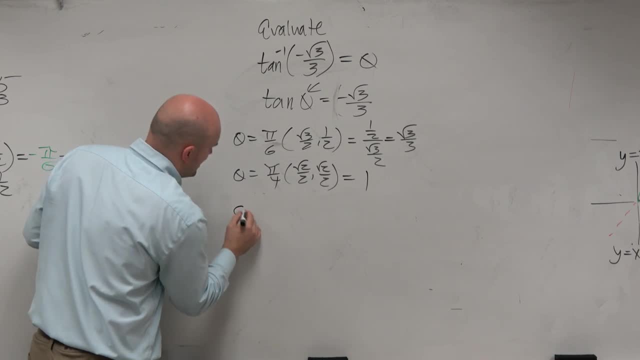 And you just kind of keep it right there, OK. And then, oh, let's just do pi over 3 real quick, Because that one was square root of 3 over 2.. Oh crap, Did I mess that up? 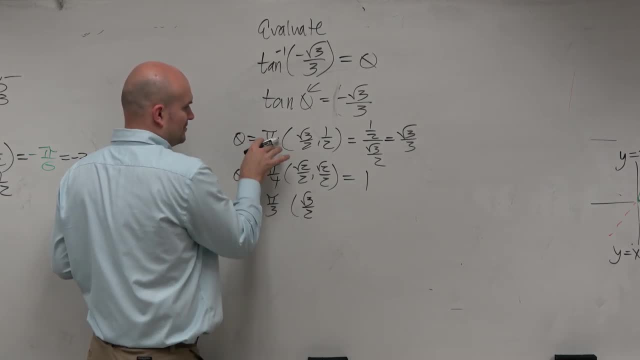 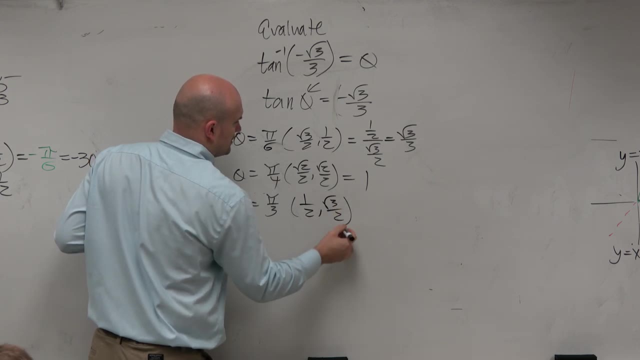 Dang it, I did. No, this one was yeah. yeah, I was right. I'm sorry I wrote this one wrong. Then, when you do this, you get square root of 3 over 2 divided by 1 half. 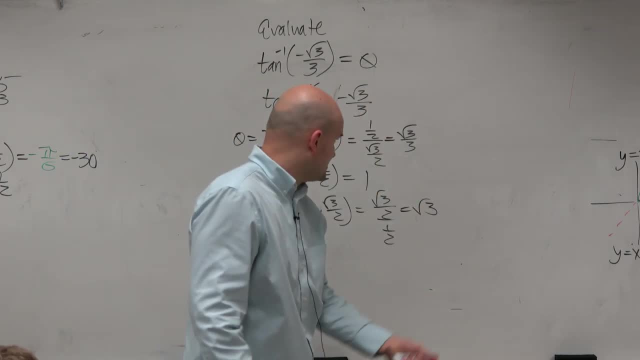 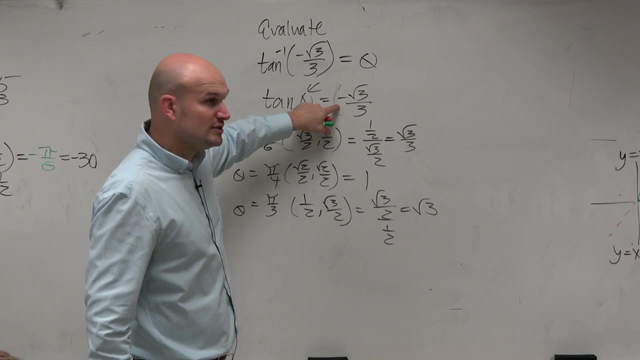 And that just equals the square root of 3.. Now, anyways, I made a long little example. Here's our angle. So we know that the tangent is going to equal. forget about the positive or negative. We know tangent is going to equal negative square root. 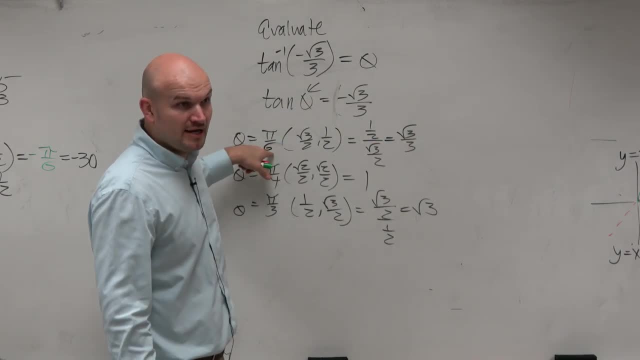 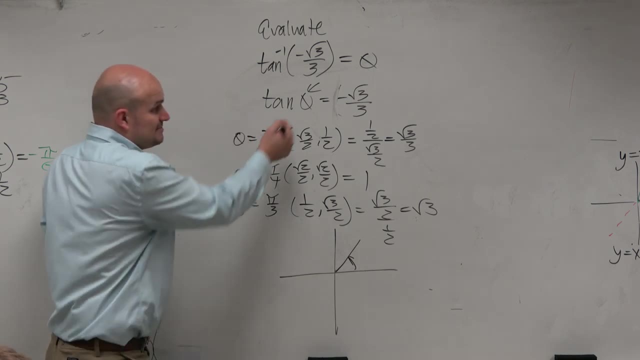 of 3 over 3 for at least a reference angle of pi over 6.. Right, So we go and look at our unit circle And we say, all right, there's pi over 3.. It has to be negative, though. 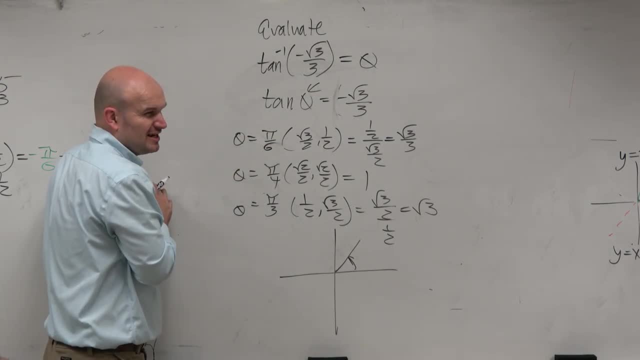 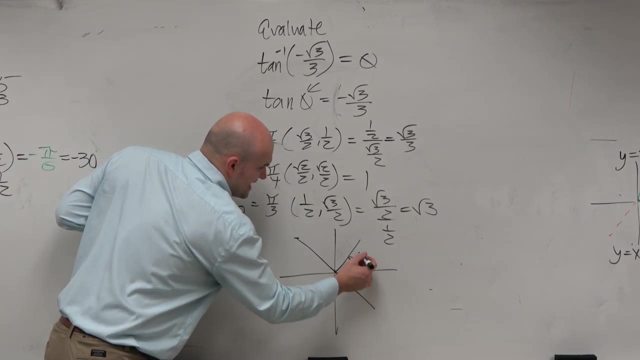 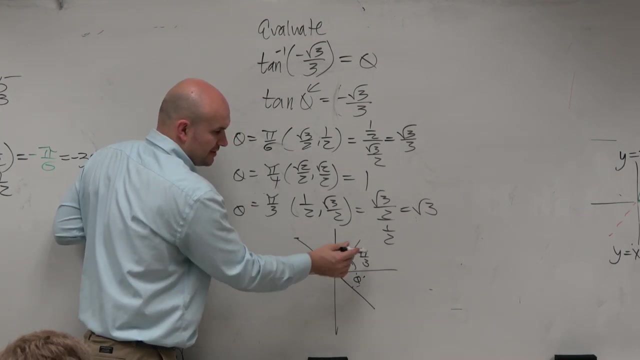 So therefore it has to be in the when is tangent negative. Second quadrant and fourth quadrant: Same reference angle. Reference angle is pi over 3, right, All these angles have the same angle. That's pi over 3, that's pi over 3, that's pi over 3.. 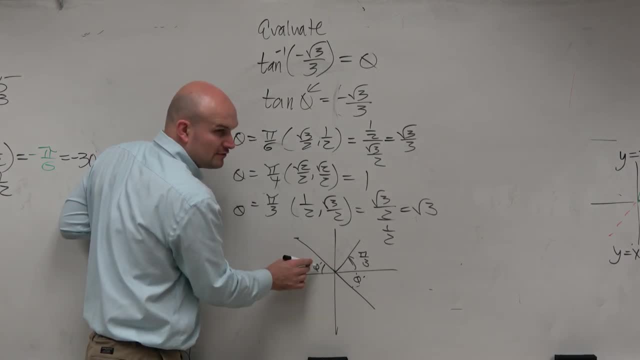 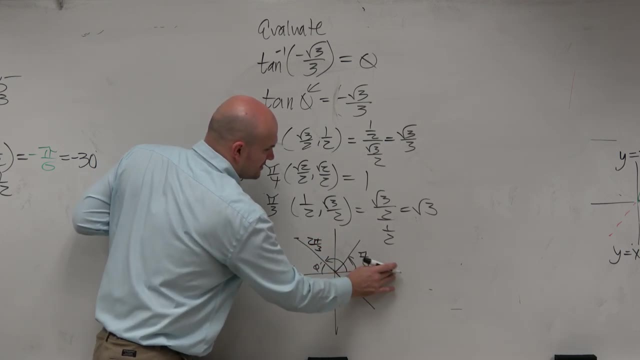 So again, guys, if halfway around the circle is 3 pi over 3 and you're pi over 3 short, then what is this angle? 2 pi over 3.. If all the way around the circle is 6 pi over 3. 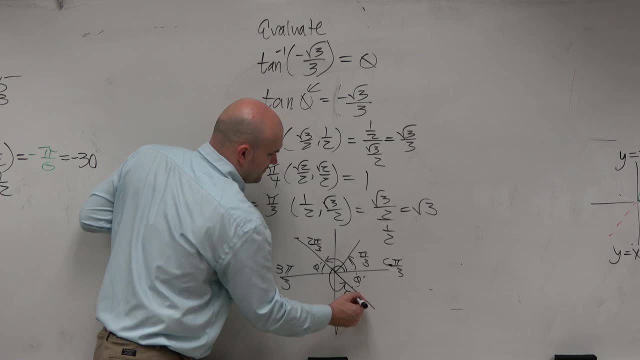 and you're pi over 3 short, then what is this angle? 5, pi over 3.. OK, But here's the problem. The tangent is restricted, or the tangent inverse, I'm sorry, is from the restriction of negative pi halves. 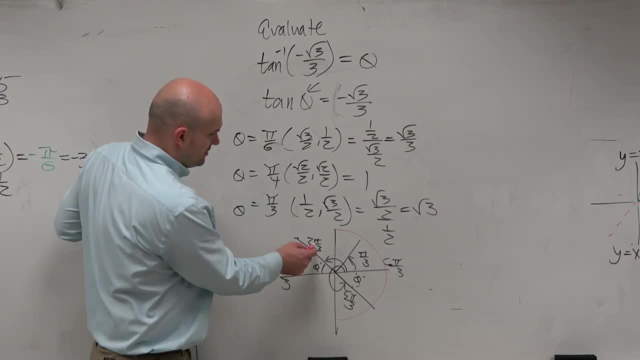 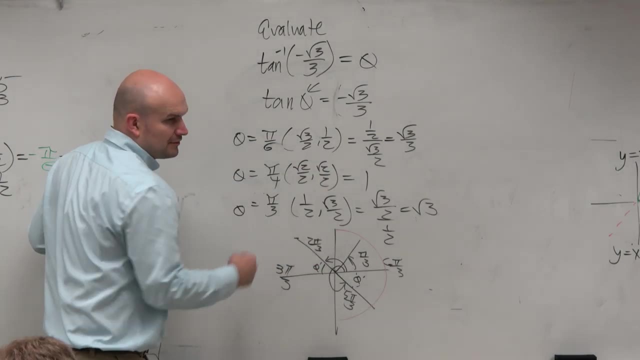 to pi halves. So does 2 pi over 3 give us negative square root of 3 over 3?? No, that's not within the restriction. What about 5 pi over 3? It gets outside of the restriction, right. 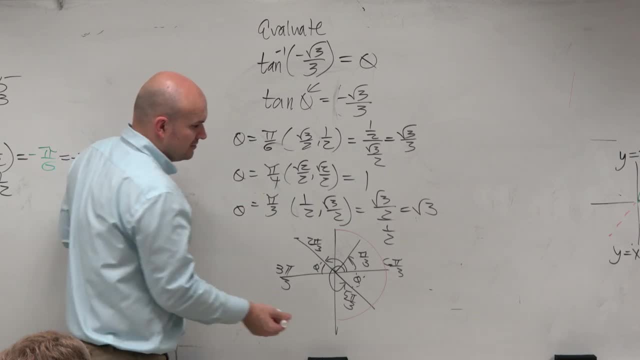 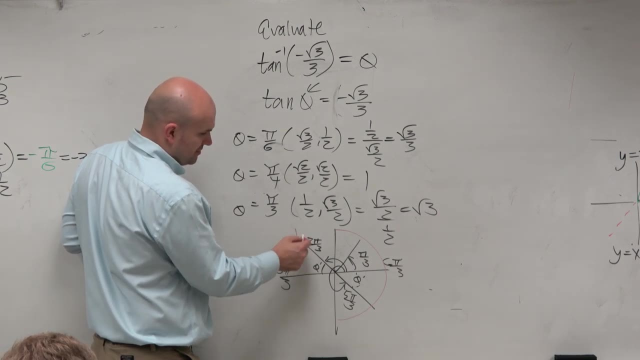 It goes outside and then comes back in. So again, we've got to find an angle, All right. first of all, no matter what angle I find, this one's never going to satisfy it right, Because it's outside of the restriction.